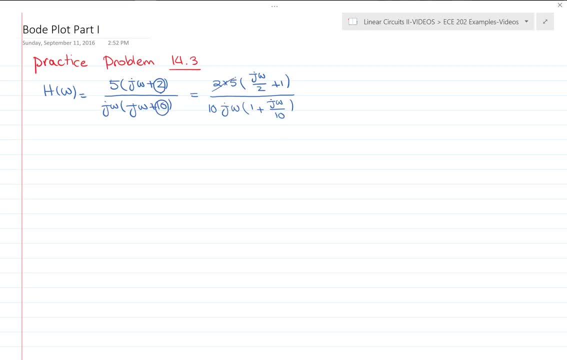 omega over 10.. And you can see that this 10 will be canceled with this 10.. So we do not have any constant gain here in this transfer function. So the final transfer function that we have to draw the body plot for is one plus j omega over two over j make. 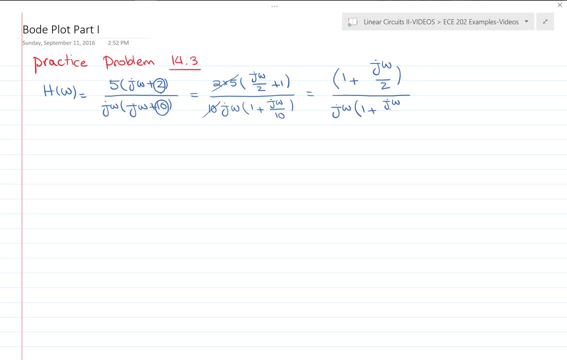 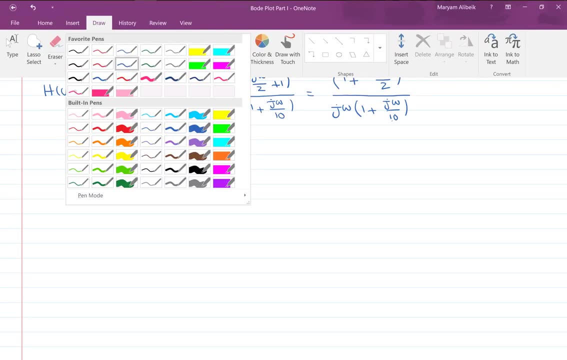 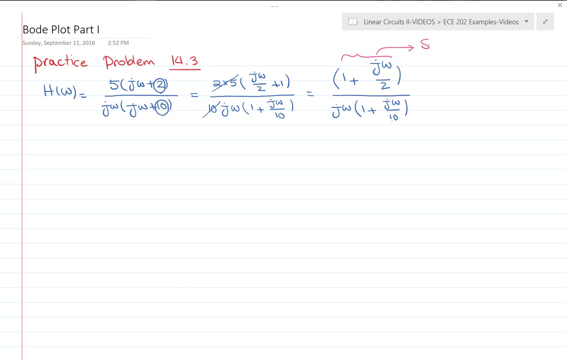 uje che omega by 1 over 1, plus j omega over 10. okay, so let's see. first for the magnitude plot, let's see what each of these factors are. so what is this factor? this is a simple zero right. and then we have the same configuration, but in the denominator. so this will be a simple pole. 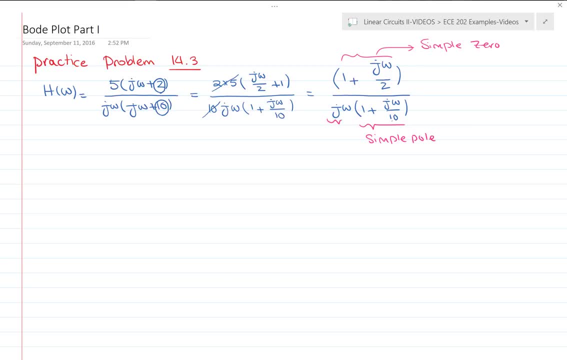 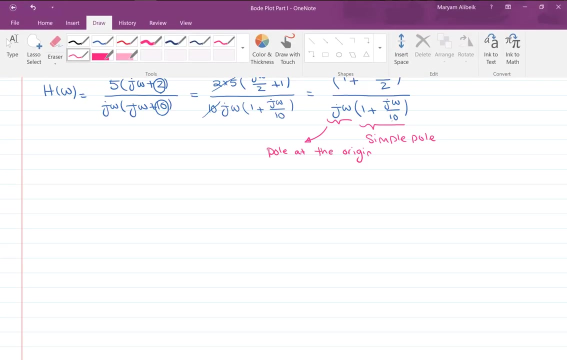 and this one one over j, omega is pole at the origin, right at the point. so now i have all the uh factors in the transfer function distinguished from each other and we can go ahead and draw them. so for the first example i'll just do that. do it on a? um plain paper. 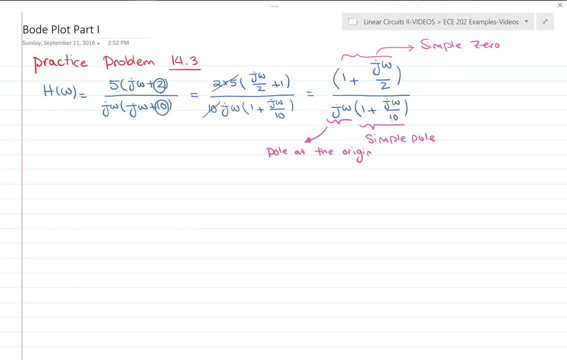 but, um, so in class i'm going to draw you. so this is trying to use the Nad fir SOC to do it on the semi-lock paper so you can see how we can draw on that paper as well, because in the exam i'm going to give you the semi-lock papers to draw. all right, so for the magnitude plot. 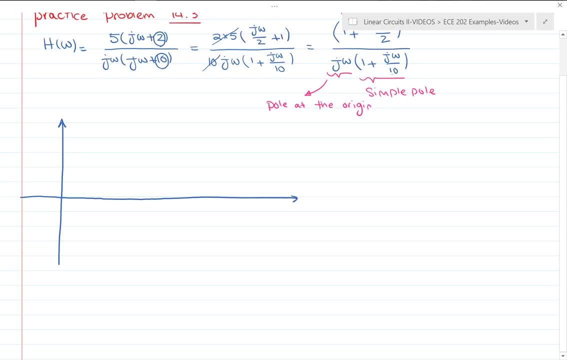 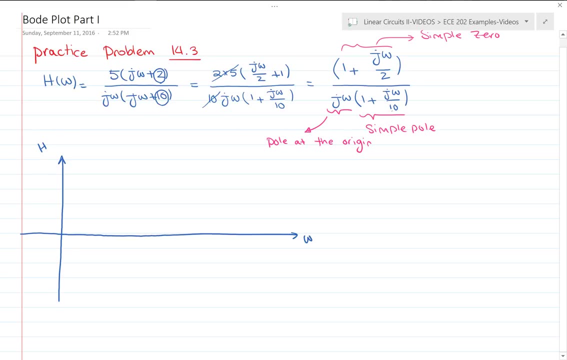 so you remember that we said in um, sketching the body plot, we have to sketch each of these factors individually and then add them graphically. so i'm going to draw each of these factors with one color and then add them graphically for finding the magnitude. plot of body plot. 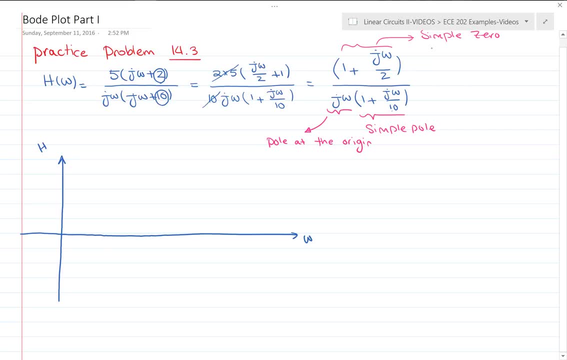 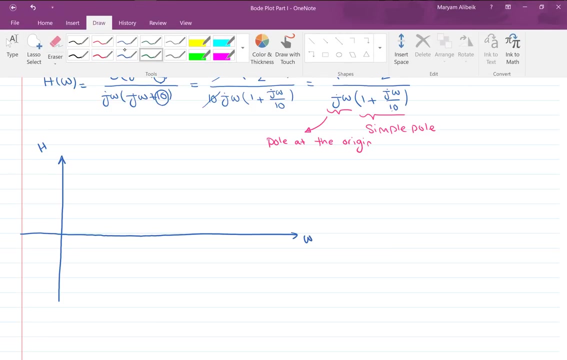 so first point is the simple zero. so if you look at the table that we have on page 623, you can see that if we have a simple zero, which is one, two, three, fourth row, it says that: oh, let me first specify the frequencies that we have here on the axis. 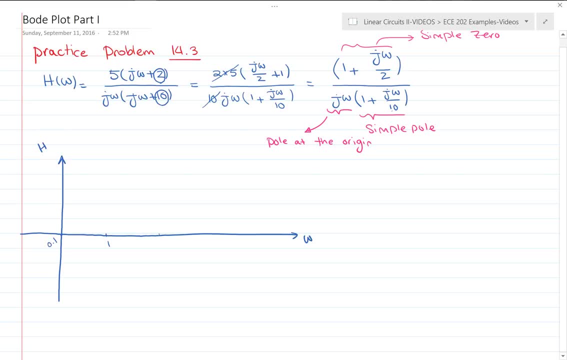 zero, point one. and then we have one ten and 100, and then here is 20 decibel, here is 40 decibels. so the good thing about semi-lock papers is that they have all of these already defined on them, so your graphs will be more accurate. all right, so the first one was a simple zero. so for the simple, 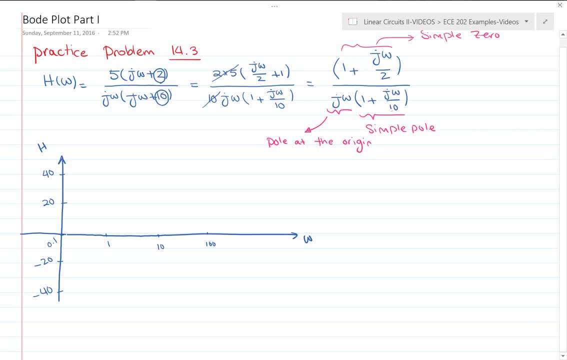 zero. we know that the plot will be zero until we specify the right number of Pokemon in every second. you can see it from here. the whole thing will be the same for every single color, so it is always 10, while 50 decibels is 20. you can see that there is still 0 here, which is 2, so 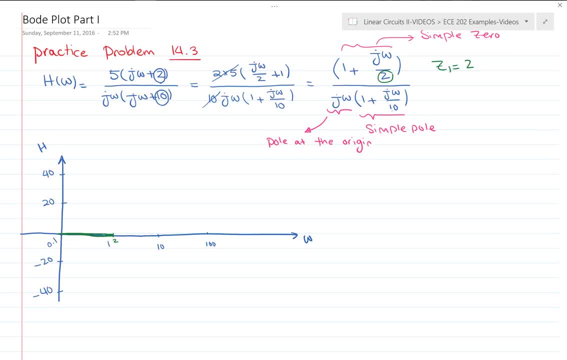 our 0 z 1 is equal to 2. okay, so if, if this is 1, this is 10, then this can be defined as 2, so it says that it is 2, So it is 20 decibels per decade. It means that from 2, from the frequency of 2 until the frequency of 20, okay. 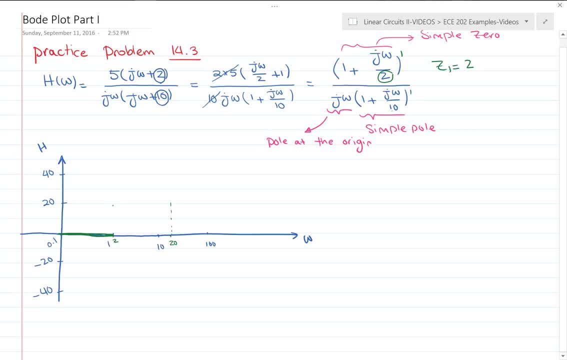 the magnitude should increase 20 decibels. So this will be our plot, And then again, from 20 to 200, it has to reach 40.. Okay, so it is somewhere over here. See, since we don't have the similar plot, it is a little hard to draw them in the exact place. 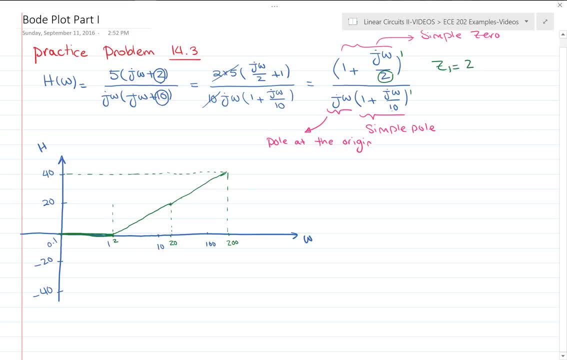 but it will be something like this. okay, So this is our simple zero. Then we can go ahead and draw the simple pole or the pole at the origin, It doesn't matter. So I'm going to draw the simple pole first. Let me change the color. 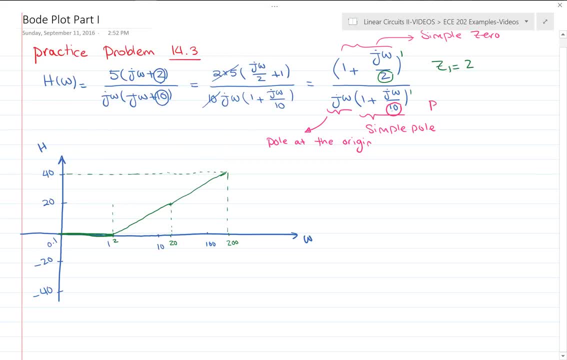 What is our pole? Our pole here, it is 10,, right, So P1 is equal to 10.. So, for the simple pole in the table, which will be row 1,, 2,, 3,, 4,, 5th row, 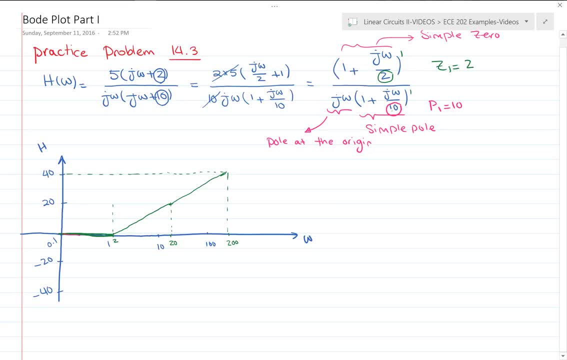 it says that the plot is equal to 0 until 10.. And then it will decrease with the slope of negative 20n. And n is equal to 1.. So it is negative 20.. So from 10 to 100.. 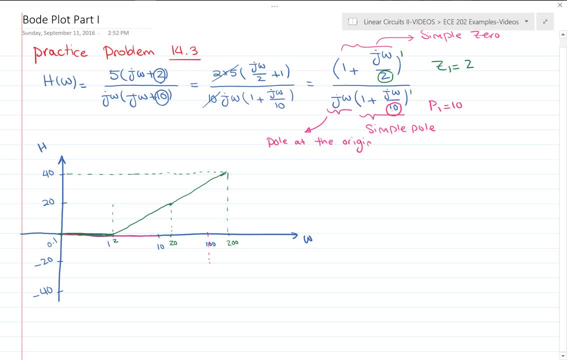 It has to reach 20,, which is here, So it's a little hard to draw exact line- And then, from 100 to 1,000, which is another decade, we have to reach 40.. Okay, so this is my simple pole. 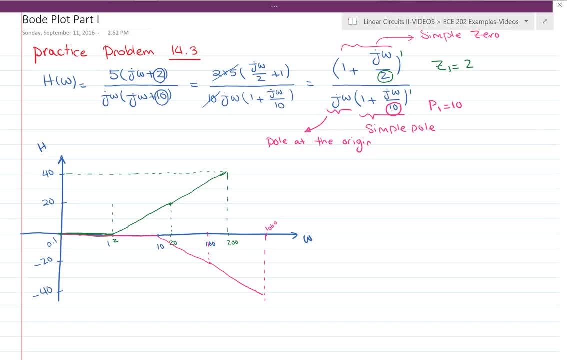 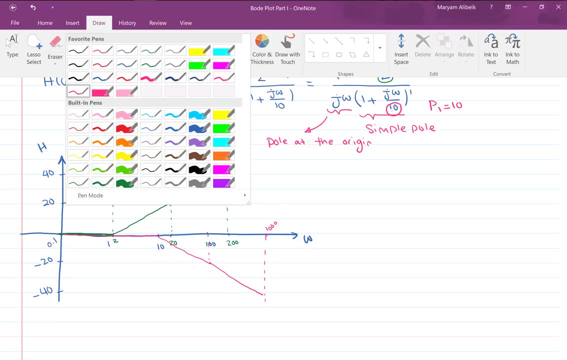 So the only thing that is left- Okay, so this is my simple pole. So the only thing that is left Is the pole at the origin, which is 1 over j omega. So let me draw it with another color, Orange. 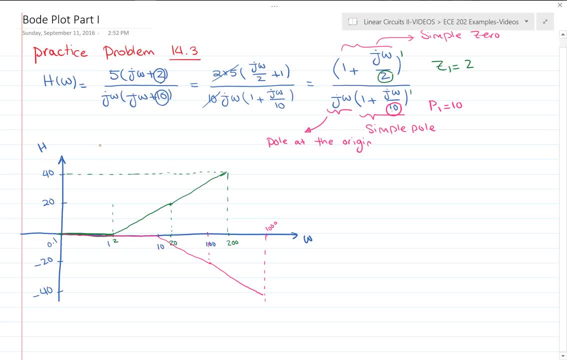 Okay, So for the pole at the origin- it is the third row in the table- You can see that the slope is negative 20 and it has to pass frequency of one. So when it is reaching frequency of one, the magnitude is equal to zero, right? 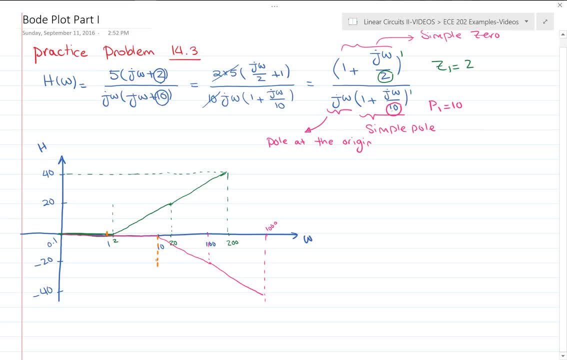 So This is 10 and then this is 20.. So this will be my plot for 1 over j omega. Okay, something like this: Okay, now we have all our plots ready. So we have 1 plus j omega over 2, which is the green one. 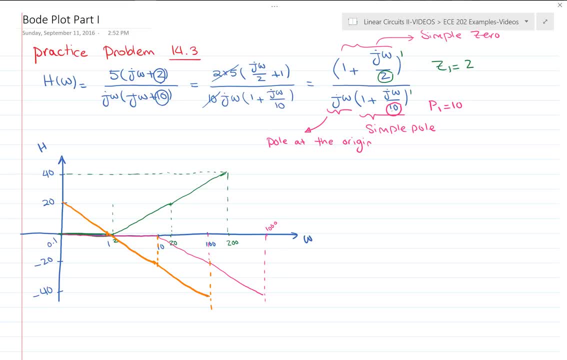 We have 1 over 1 plus j omega. Okay, 1 plus j omega over 2 to 10, which is the pink one, right, and then we have 1 over j omega, which is the orange one. so now we can go ahead and add these graphs. 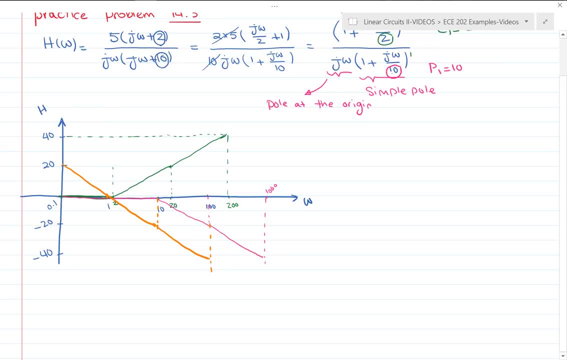 graphically. so you haven't seen this part before because the previous ones were like the things that I just talked about. all right, so let's add them graphically. see, the frequencies that something happens in the Bode plot are the frequencies that these plots will will meet each other at those places. so one of them is frequency of 1 another. 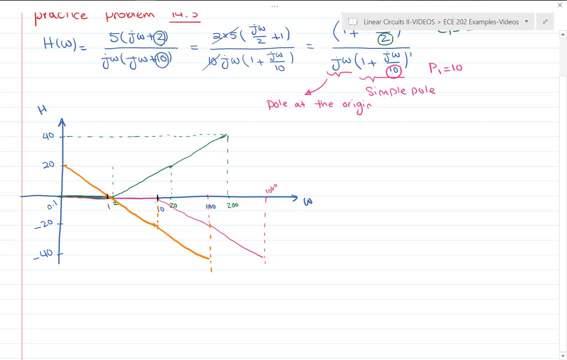 one is the frequency of 10, and I think that's it. yeah, that's it okay. so let me go ahead and add these graphs and then we can go ahead and add these graphs and draw these. it's not necessary to define these frequencies, but it will be easier. 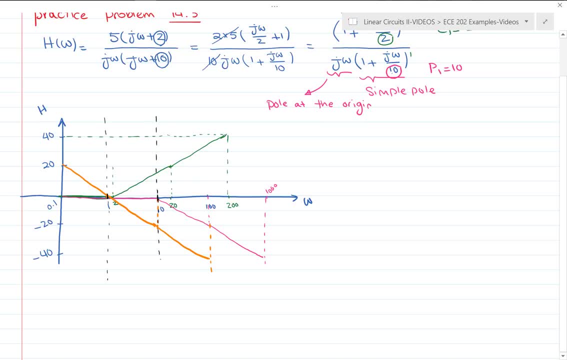 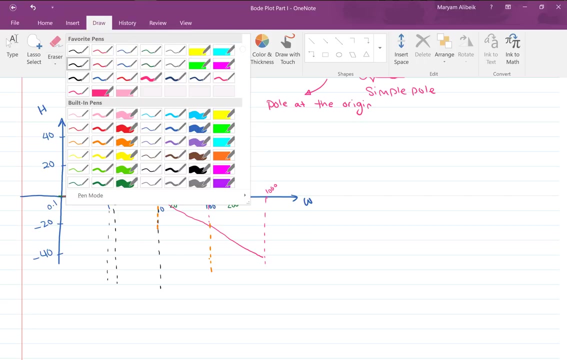 for you to find out where the Bode plot has to change. so, oh, and also one at two. right, they may or may not change at these frequencies, but if you define them, then you will work more accurately. and let me change this plot here. it's a little too thick, so I get confused. 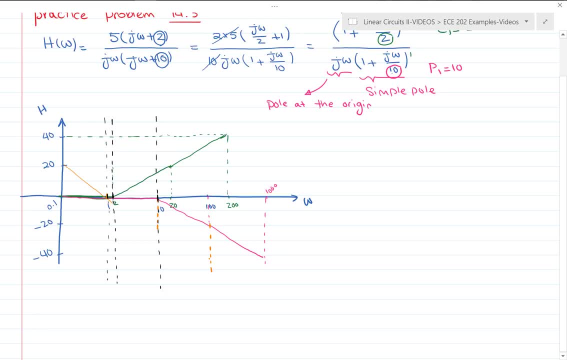 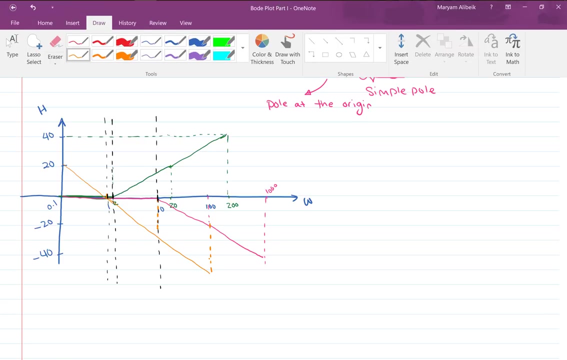 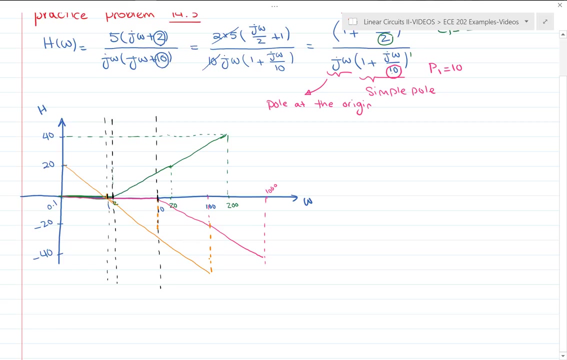 okay, so from 0.1, from the frequency of 0.1 until the frequency of 2, you can see that we have the green plot is 0, the pink plot is 0, but the orange plot is 20 and it is decreasing with the slope of negative 20, right? so if you add, 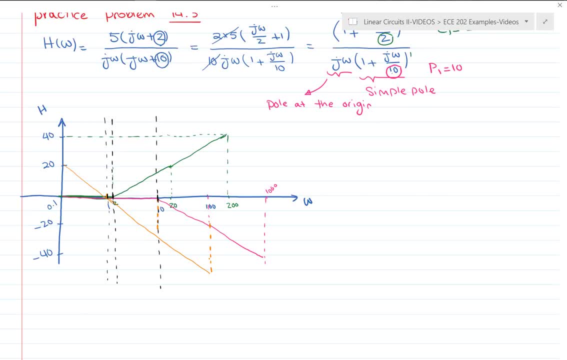 these plots together. if you add each point of these plots together, you will get the same plot as this one right, because the other two plots are equal to 0, so they don't have any effect on the Bode plot. then, when we reach the frequency of 2, you can see that the orange plot is. 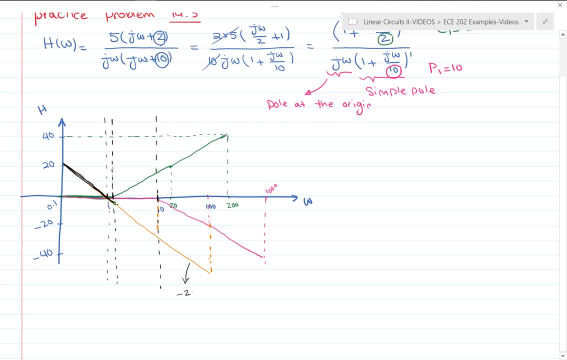 decreasing with negative 20. I will write here: negative 20 decibel per decade. the pink plot it is 0, but the green plot it has the slope of 20 decibel per decade. so what will happen? here? we have 1 negative 20, we have 1 positive 20. so if we 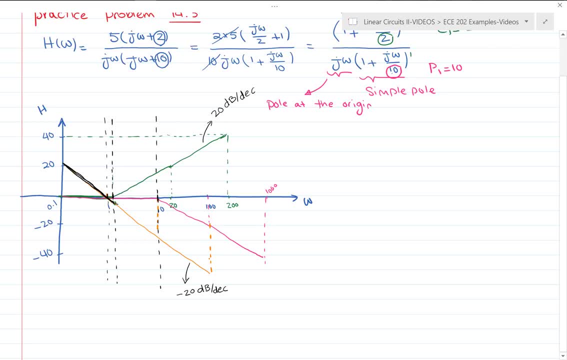 add them together, it will be 0. so we're going to have a plot with slope of 0, okay, until we reach frequency of 10, and then, at the frequency of 10, we will have all three waveforms, all three plots. right, we have negative 20 and again the 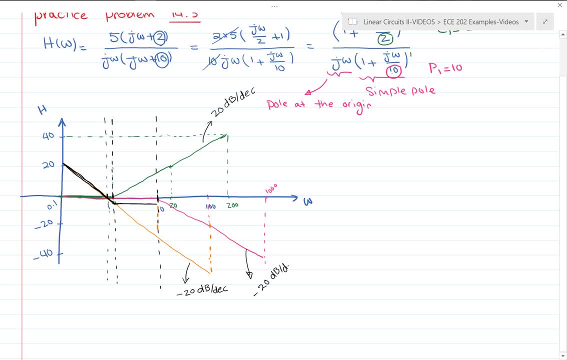 pink one is negative 20 decibel per decade, and then we have the green one, which is 20 decibel per decade. so we're going to have 20 minus 20 minus 20. these will be negative 20 decibel per decade. so we're going to get a plot. 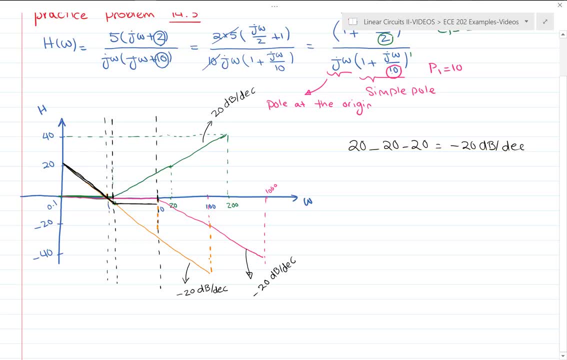 which is decreasing with the slope of negative 20 per decade, and from this frequency on, we do not have any other changes. so, as you can see, we add these three plots graphically and we got the black one, which is our body plot, the magnitude body plot, yes. so let me just 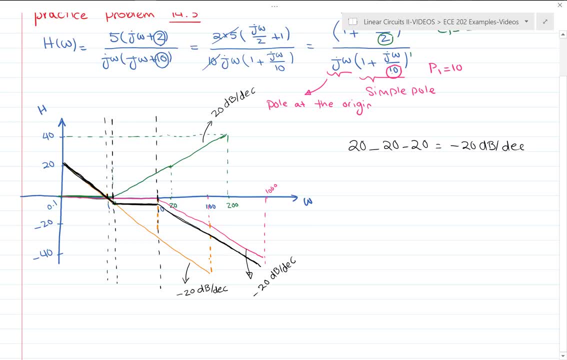 make it a little thicker. so the black one is what we are looking for. so in the exam, for sure you have to show all these steps and for sure all of them has some points: the partial credit. but to get the full credit you have to be able to. 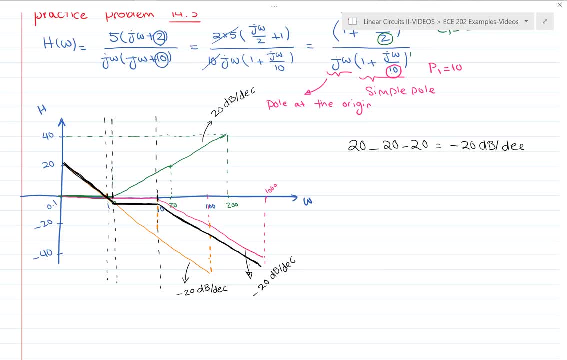 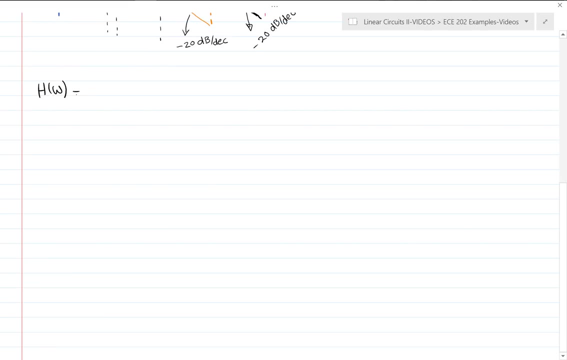 sketch this black one as well. so this was the magnitude plot. let's go through the phase plot as well for this transfer function. so the transfer function was: H of Omega is equal 1 plus J Omega over 2 over J Omega, multiplied by 1 plus J Omega over 10. okay, so this time we have to look at the phase plots. 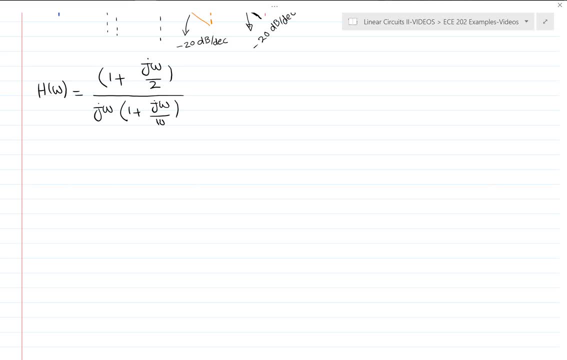 in table 14.2.. three, so you can see table fourteen, point three. it has three columns. first one is the factor, so the factors that we have in the transfer function. second one is the magnitude plot and third one is the phase plot. okay, so go ahead and look. 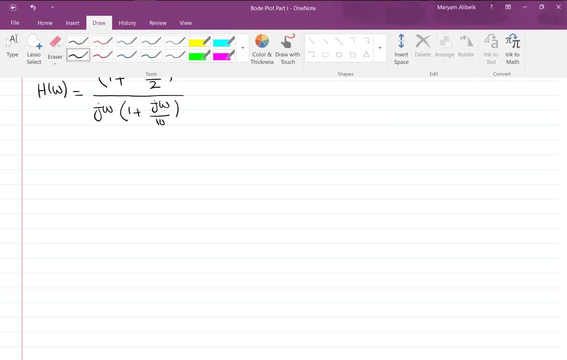 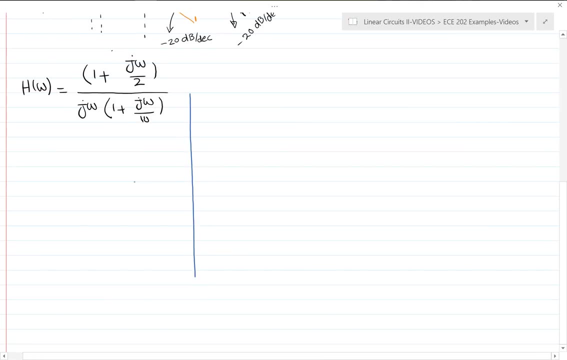 at the phase plus. alright, so let's draw the phase plot for each of these factors here in our transfer function. so Omega Phi, zero point one, and then one, ten hundred and thousand. why am i writing this like? why is the intervals from zero point one to one, one to ten? because frequency is increasing in. 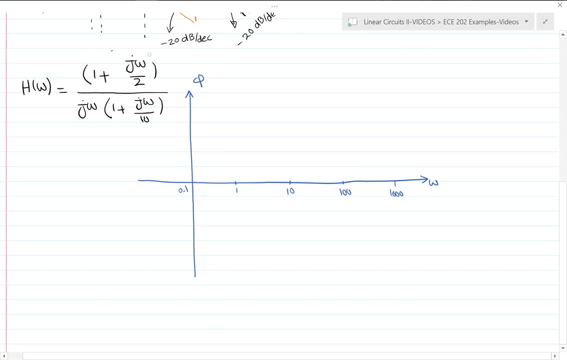 depth, second in bode plot, don't forget that. so let's start from one plus J, Omega over two, which is a simple zero, which is the fourth row in the table. you can see that the phase plot is going to remain and it will be zero until Z over ten. sorry, I. 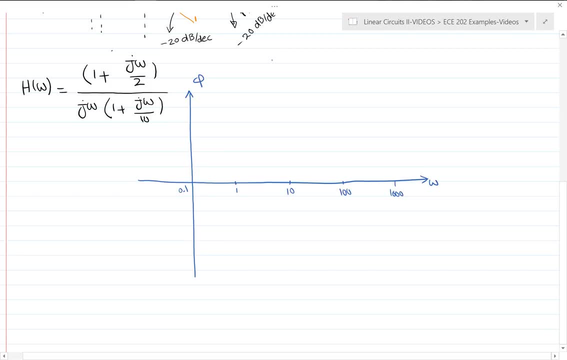 was looking at the wrong plot so what is the over ten C one is equal to two so Z one over ten will be equal to zero point two right so it says that if this is two zero point two it will remain at zero point two correct and then at ten � immigration let's open the goods 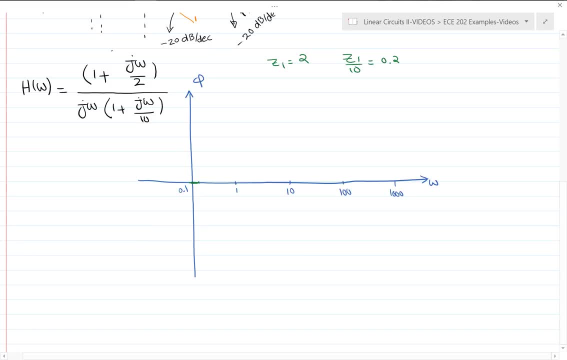 at ten Z, which is what is ten. Z is two multiply by ten, which is twenty. okay, so at twenty it has to reach ninety. N and N is equal to one. and then up here you'll get, if we something like that, because go to the third group in the whole line, right now it contains the number of times a two, so we can do not get the number of times a two forward as well to find zero point two. it's ok, so it'll remain at your right and you'll get to the value at 10 z. one two is 0.2, right, so it will remain 0.2, which is what is 10 z, which caught, is 2 multiplied by 10, which is 20. okay, so at 20-one, so that's 25?'. 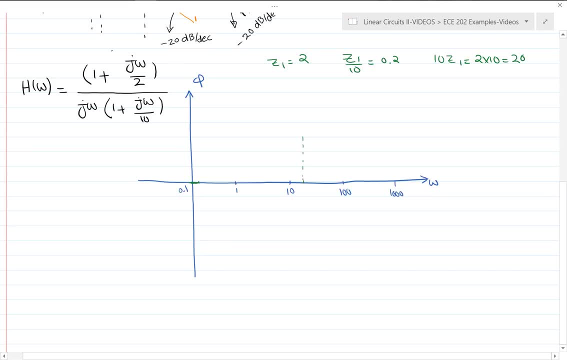 90, n and n is equal to one. so this is my plot, right, so from 0.2 to 20.. okay, so how can i find the um slope of this plot before it reaches 90.. see, from 0.2 to 20, it's not one decade, it is two decades. right, first, from 0.2 until 2. 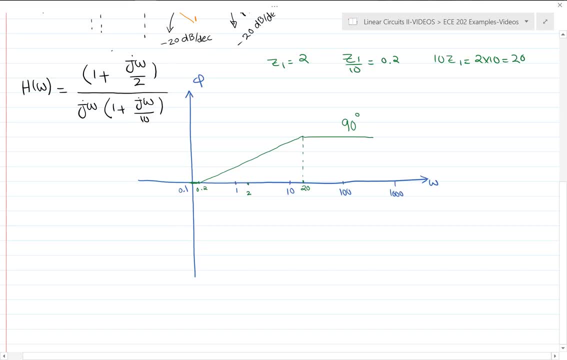 is one decade, and then from 2 to 20 is another decade. so in two decades. so in two decades we reaches, we goes from 0 to 90. so we can easily say that in one decade we would go from 0 to 45 degrees. okay, so this plot: here it has slope of 45 degrees per decade. so for sure, here, 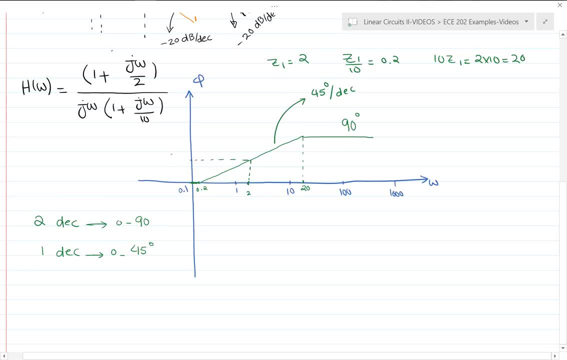 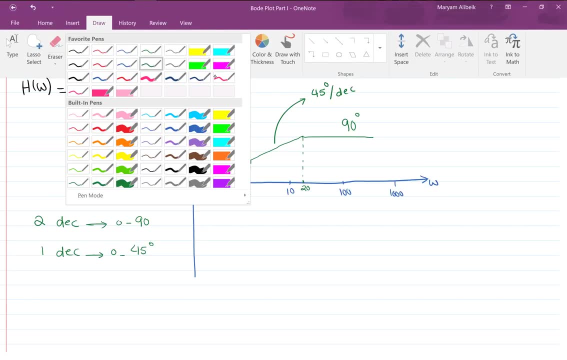 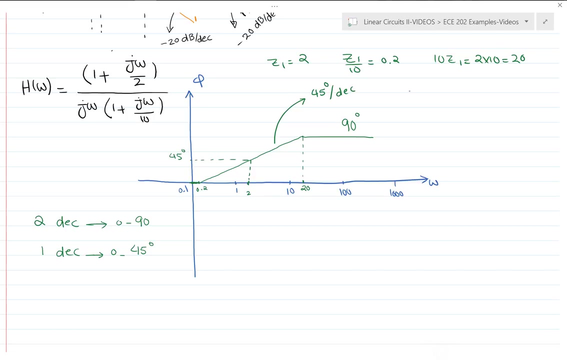 it's not accurate here, but at two we're gonna have 45 degrees. okay, now let's go and draw for the pole. so one over- i'm sorry one- plus j, omega over 10. so p 1 is equal to 10 and um. p 1 over 10 will be equal to 1 and 10 p 1 is equal to 100.. okay, so 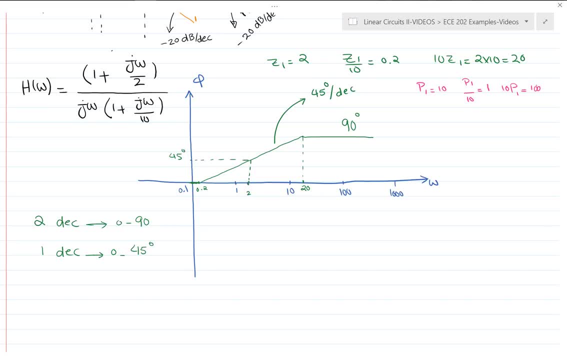 um one, two, three, four. fifth row in the table, it says that the plot should remain zero until p over ten. p over ten is equal to one. so until the frequency of one my plot will be zero. and then it has to decrease and reaches minus 90 degree at 10 p. so 10 p is 100. 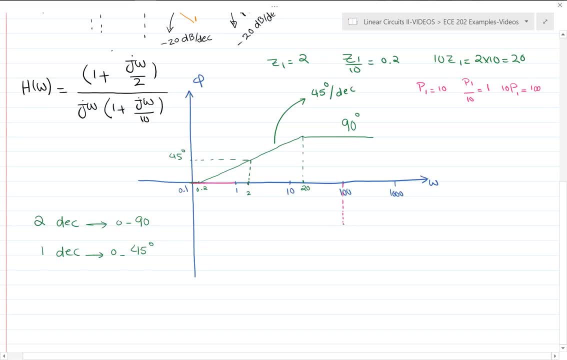 so in 100 it has to reach negative 90. okay, if i want to be consistent with the one that i drew for zero, i have to do this. um, it goes down and we know that this one is the same as the other one, only the negative. so minus 45 degrees per decade, okay, and then we have to draw. 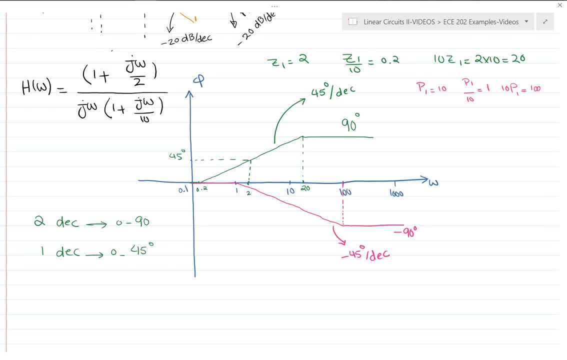 the face plot for um the pole at the origin, which is easy. it is negative 90.. so let me draw it with print: it is negative 90.. okay, so these three are um separate plots for um each factor, and now i have to add them graphically, so let me. 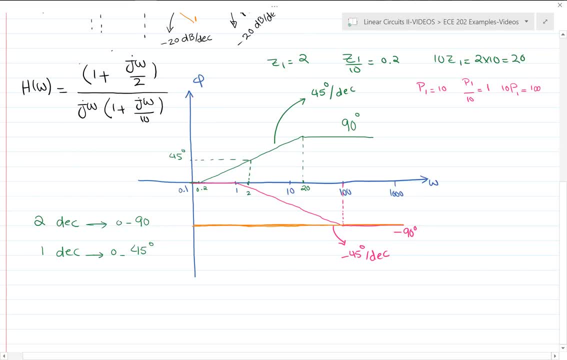 specify the frequencies that something is happening in them. so it is 0.2 which is here. so, as i said, there might be not and not nothing, or um, yeah, for we can't. we can't say that's good, but for sure, at these frequencies the body plot will change, because if the, for example, other ones, 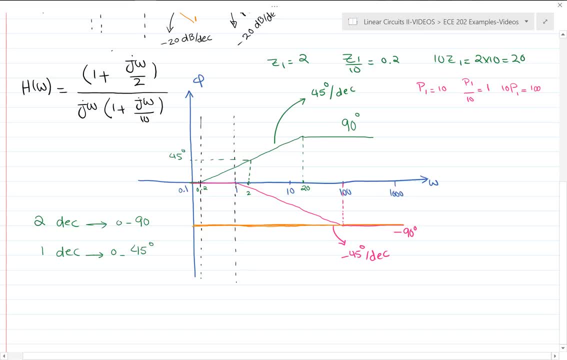 are zero, then nothing will happen. so this goes to: and then 20 is another frequency, and then 100. okay, so let's see what is happening here: 0.1 until 0.2. the green plot is 0, the pink plot is 0, but the orange plot is negative 90. so we're. 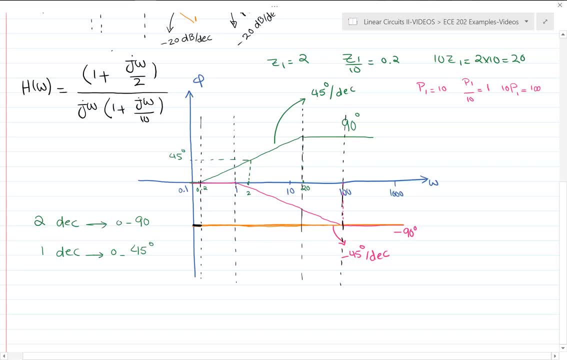 gonna have this, because negative 90 plus 0 plus 0 will be negative 90.. then from 0.2 until 1, we have the pink one is 0, so it doesn't have any effect, but we have a green one with negative, uh, with. 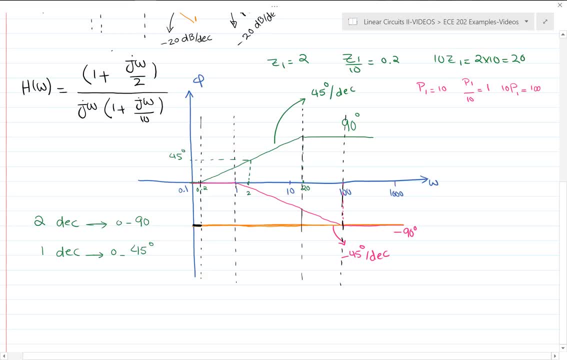 positive 45 degrees per decade, while we have the orange one in negative 90. okay, so the green plot will be shifted down here, right, okay, and then from one to two, or see from, for example. here is the example that i said. they may not change. so from 1 to 2 and from 1 to 20, we have 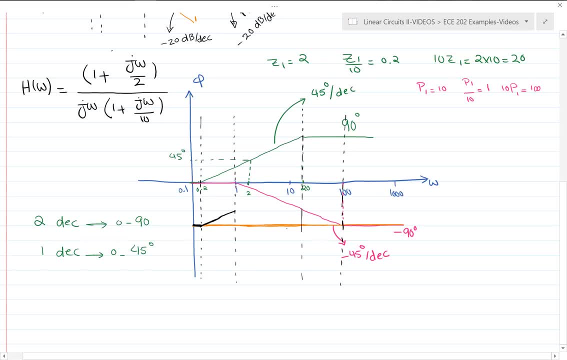 the same three plots. so the green plot, the pink plot and the orange plot are not changing in the interval of 1 until 20.. right, so we have the green one with 45 degrees per decade, we have the um pink one with negative 45 degrees per decade, and then um the orange plot, which is at negative 90. so 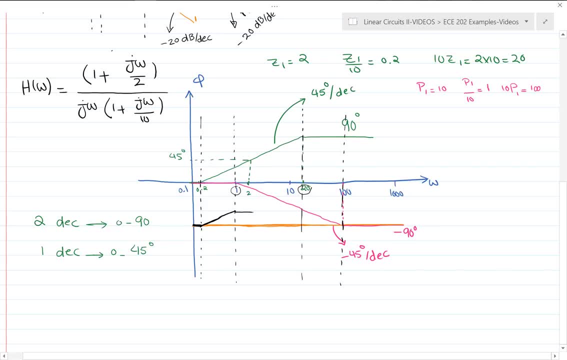 those two will cancel each other. so we're gonna have the same slope as we have for the orange plot right, and then from 20, 0.1 to 0.2, we have the green plot at 90 and we have the orange plot at negative 90 and then the pink plot. 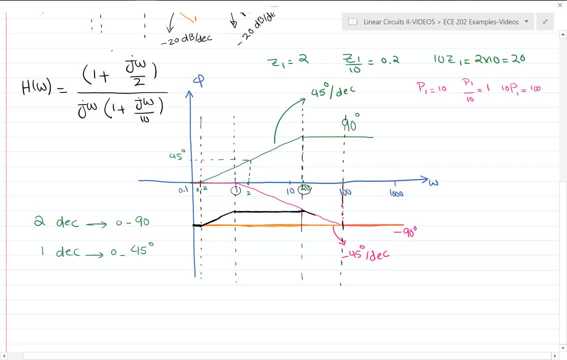 is negative 45 per decade. so it goes down like the pink one. okay, and then at um 100 we're gonna have negative 90 for the pink one, negative 90 for the orange one and positive 90 for the green one- green one. so we're going to have negative 90 for our body plot. so for the face plot you may be a. 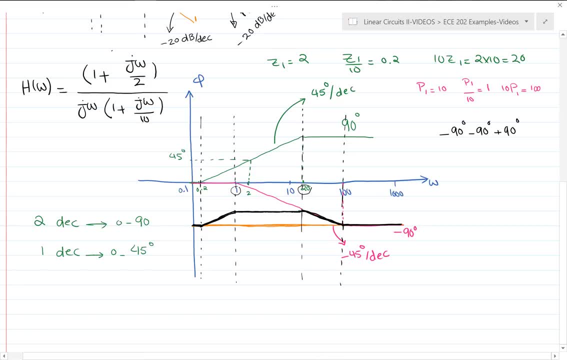 little confused in the beginning, but i'm going to talk more about it on tuesday because i want to draw it on the semi-lock paper so you can see what's going on better. okay, so please watch these videos before tuesday class because, um, i want you to have an overview on what the body plot is and how we can draw them. thank you,